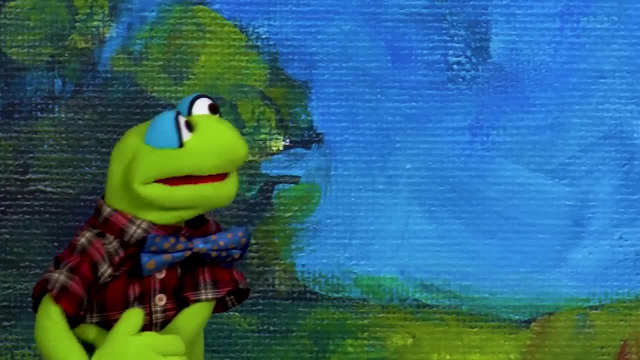 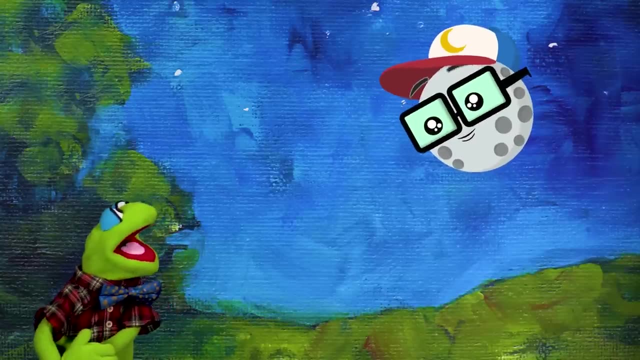 Oh, I got a lot to do. Fine, I like your singing. Ah, who said that? Up here, It's me, the moon. Oh, wow, the moon, You were listening. Yeah, I'm always out at night. 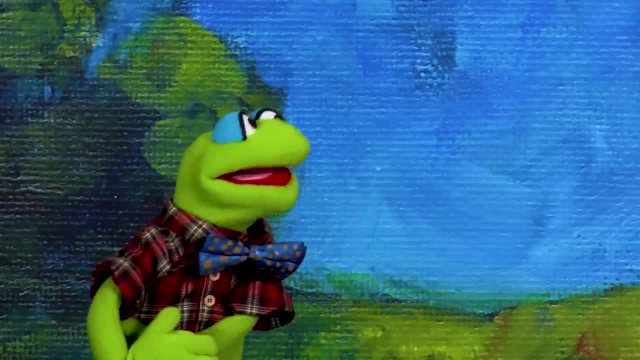 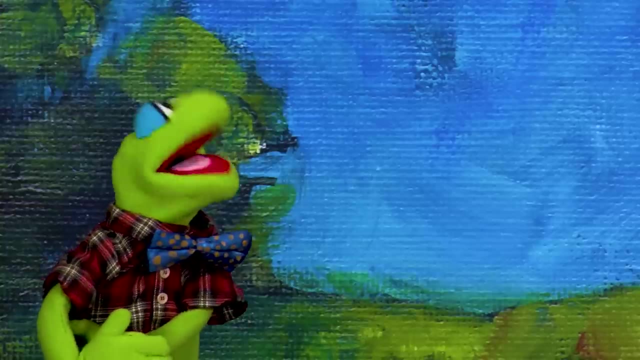 That's amazing. I see you all the time. Hey, what's your deal? anyways, I'm a big rock that orbits around the Earth. Wow, Wait, what do you mean? orbits around the Earth. Earth's gravity has a hold on me and keeps me from flying away. 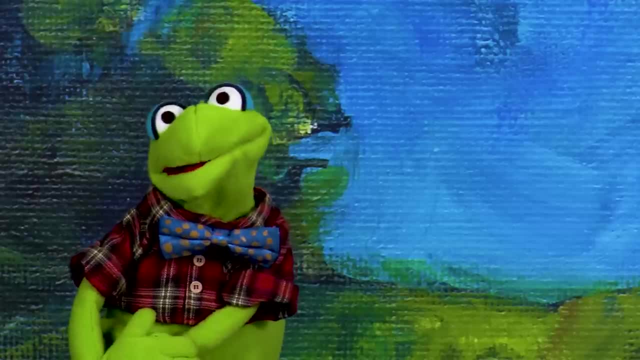 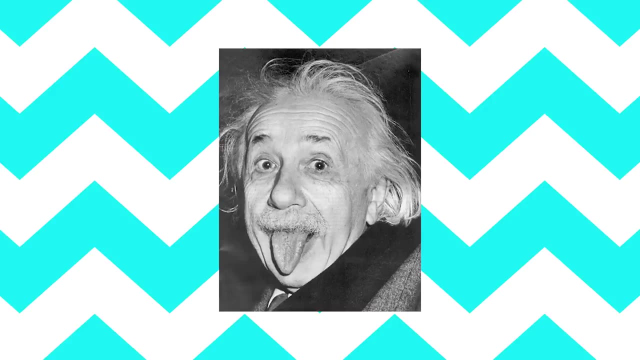 So I go around and around the Earth. That sounds complicated. It is Albert Einstein talks about it in his theory of general relativity. Albert Einstein, I like his hair, Me too. How long does it take for you to orbit around the Earth? 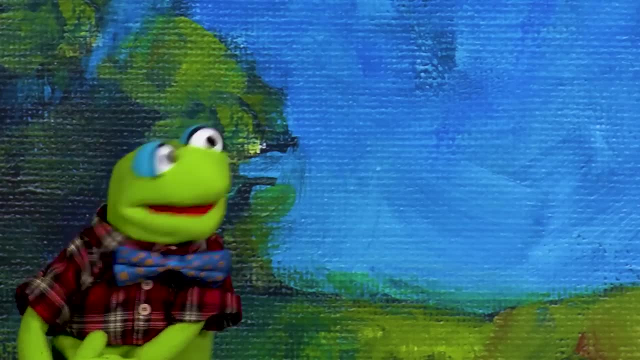 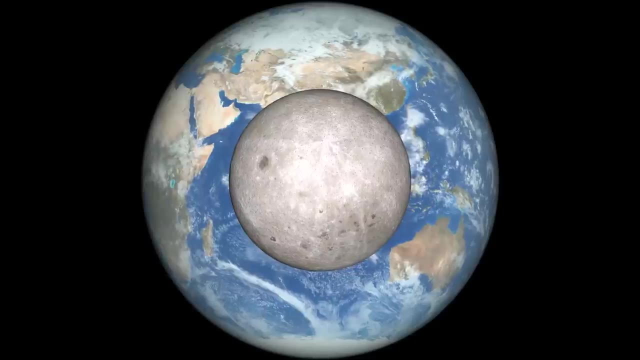 About 28 days. Wow, that's almost a month. Yeah, Sometimes when I see you you're bright and full, Then other times you're only a sliver. Why, Well, I'm moving around all the time, orbiting the Earth and orbiting the Sun. 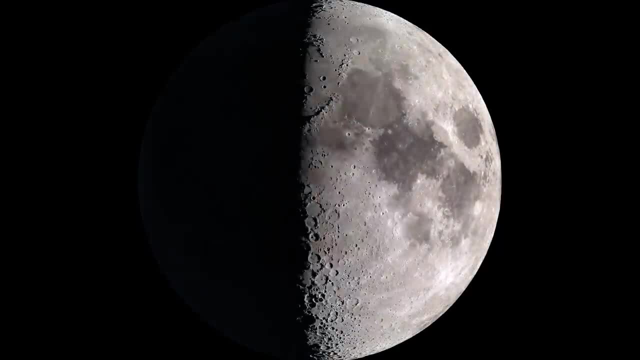 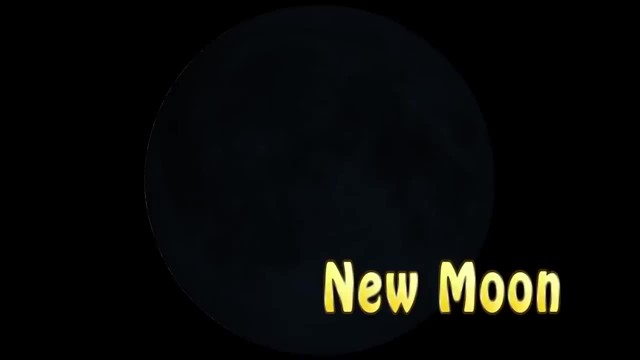 Depending on where I am, the Sun only lights up part of me. Yeah, As I move around, parts of me move into the sunshine and look bright. When I'm all dark, I'm going to look bright. When I'm all dark, I'm going to look bright. 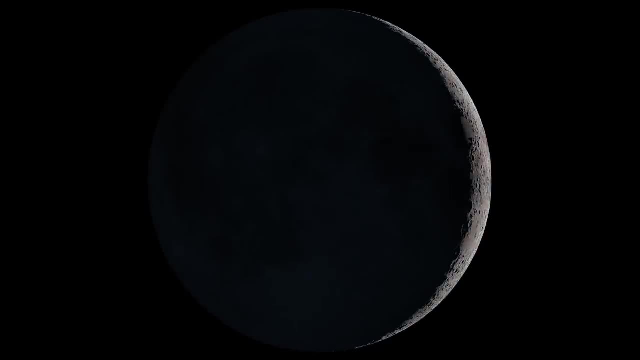 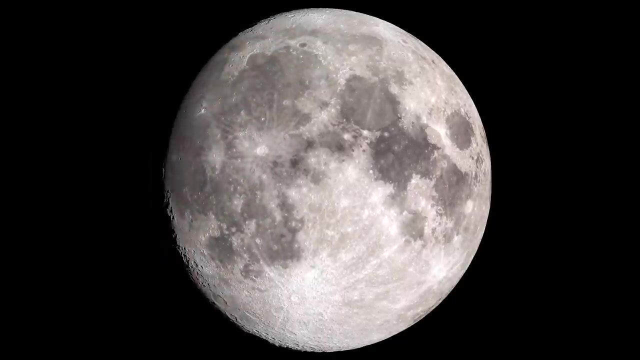 That's called a new moon. Soon I move into the sunlight a little bit And now I'm a crescent moon. I'm waxing. That means I'm growing. Now I'm all bright all over. I'm a full moon. 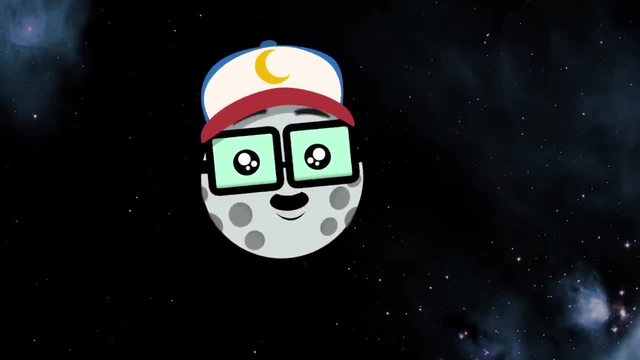 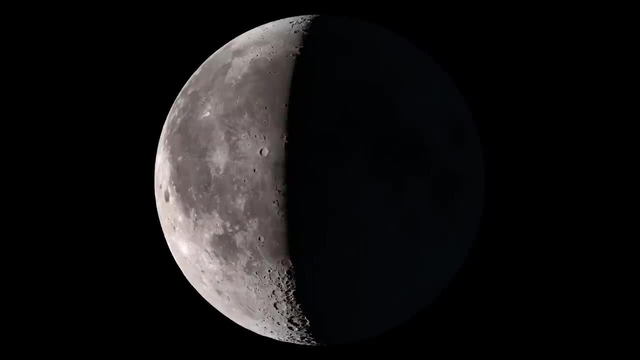 Did you know? I'm not glowing on my own like a star. I'm reflecting light from the Sun. Now I start to get smaller. I'm waning. That means I'm shrinking. I'm a crescent again. Now I'm back to being a new moon. 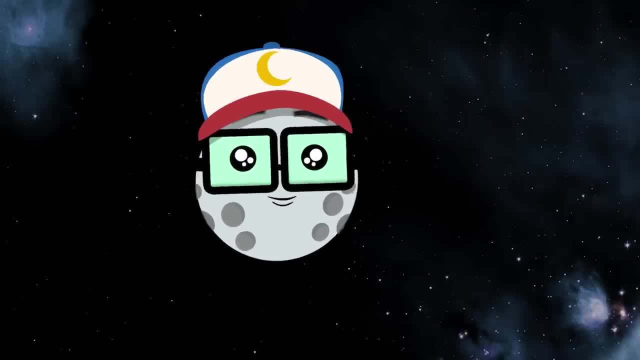 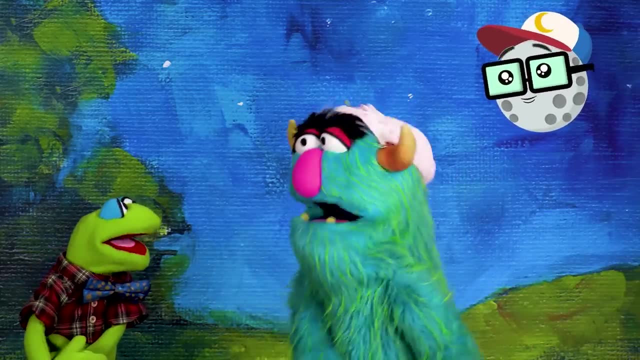 It takes about a month to see all these phases of life. I see all these phases of the Moon. What do you think, Leonard? Wow, that's amazing. Leonard, I told you to be quiet, Crump, I have company over. 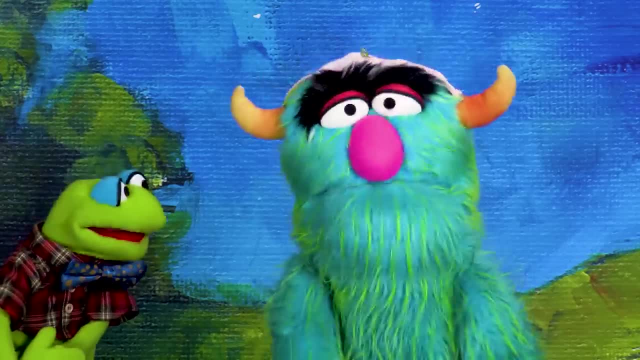 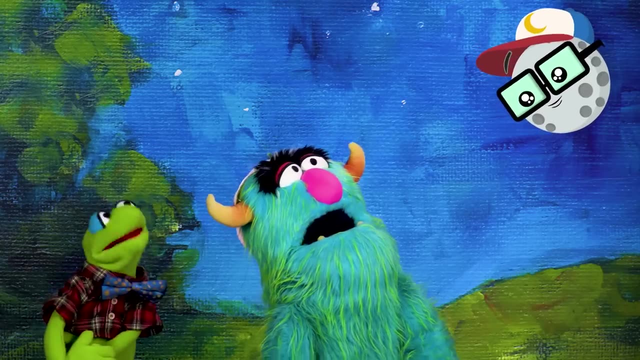 Ooh, you have company. Who would come here at this hour? Hi, Who said that? Who said that? It's me, the Moon, Isn't the Moon amazing? Ah, whatever, You're not that special. I see you all day. 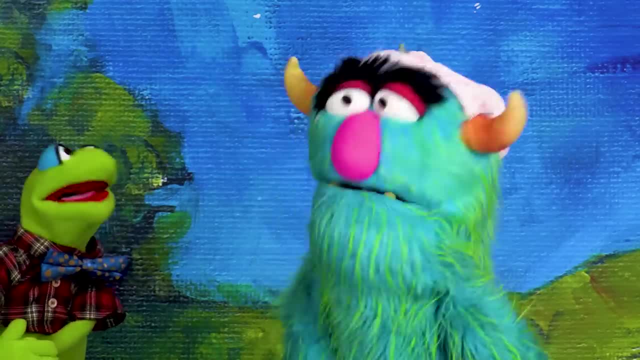 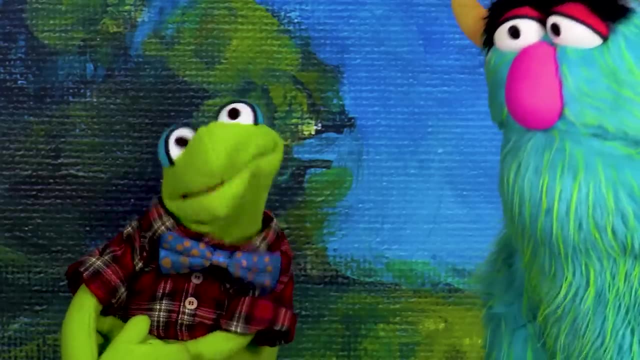 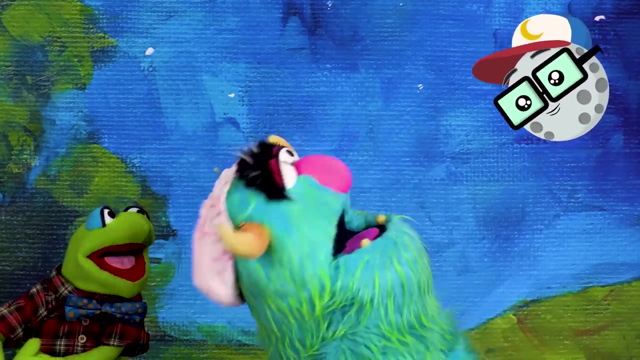 Sure I am. Plus, I hear other planets have moons too. That's right. Some planets have more than one moon. Jupiter has at least 67!. See, You're a dime, a dozen buddy. What makes you so special? I'm special because I'm Earth's moon. 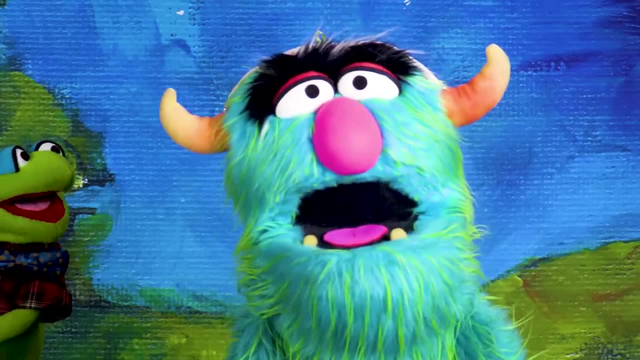 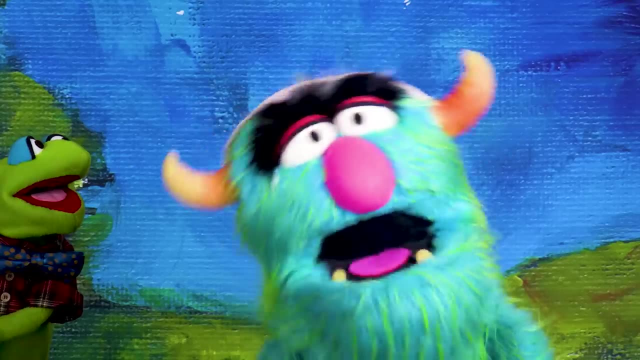 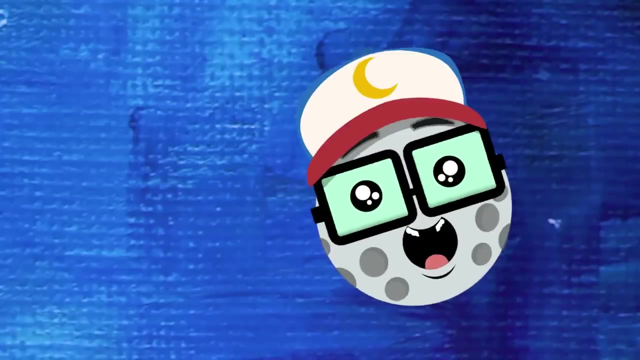 You look like you're full of holes. Are you made out of Swiss cheese? No, those are my craters. Cheddar cheese: No. Gouda cheese, No Mozzarella. I'm not made of cheese. Then how do people on the moon eat pizza? 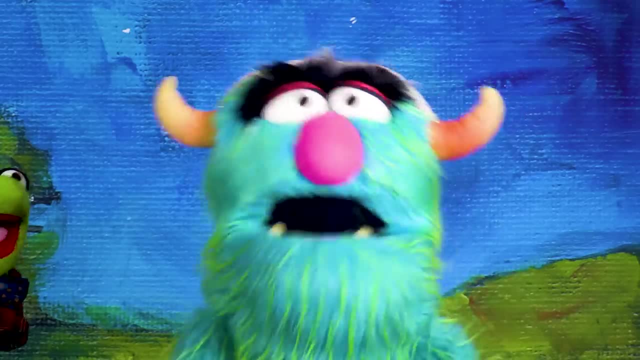 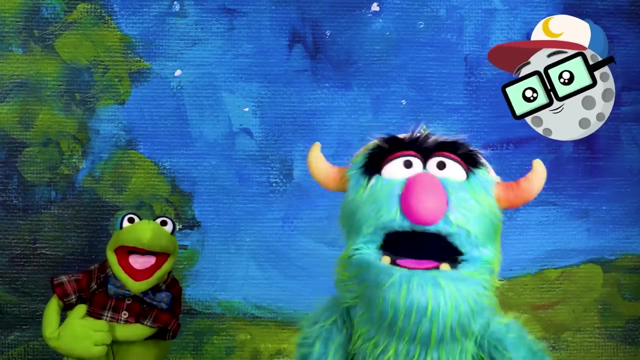 There are no people on the moon. I have no atmosphere. No atmosphere, Yeah, and And what? I don't have any food and water. What? No food. My refrigerator's more interesting than you. Hey, I'm interesting. People have visited me. 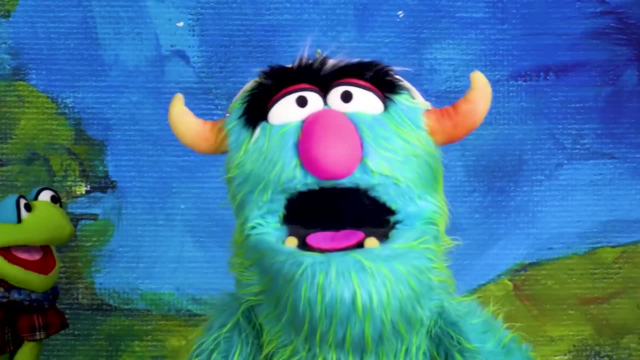 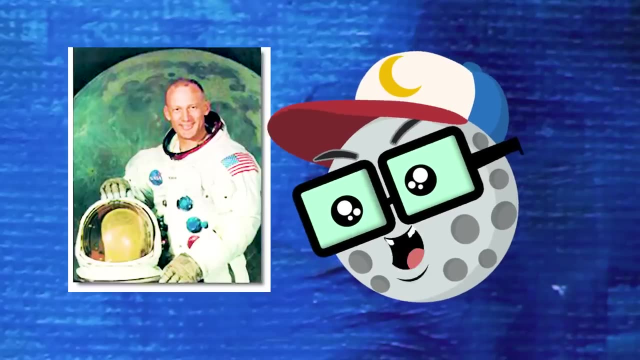 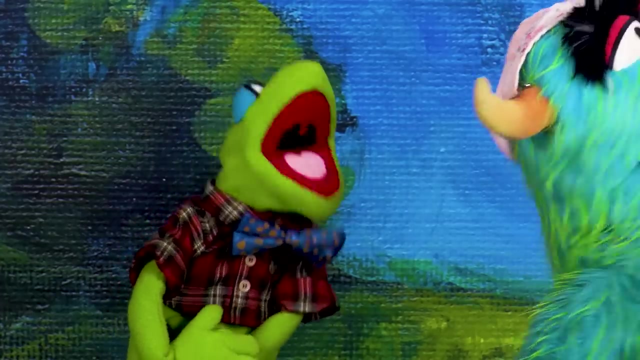 Like who Craterface. The first two people to visit me from Earth were Neil Armstrong and Buzz Lightyear. No, Buzz Aldrin, Oh, I like Buzz Lightyear. That's incredible. Can I come visit you, Moon? I'll bring my own food and water and I'll borrow a space suit from NASA. 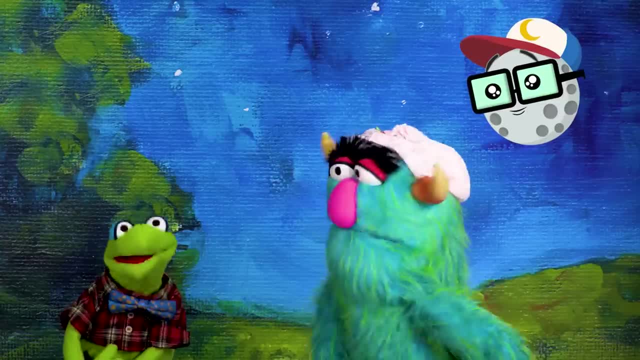 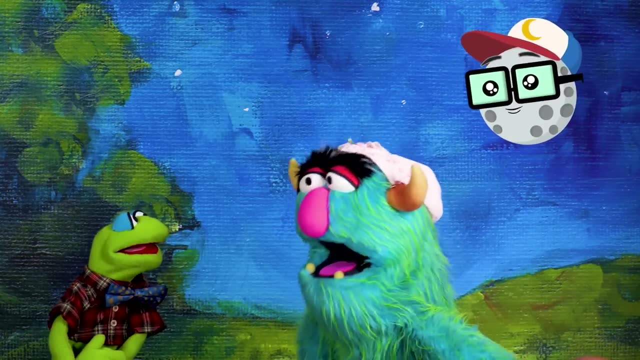 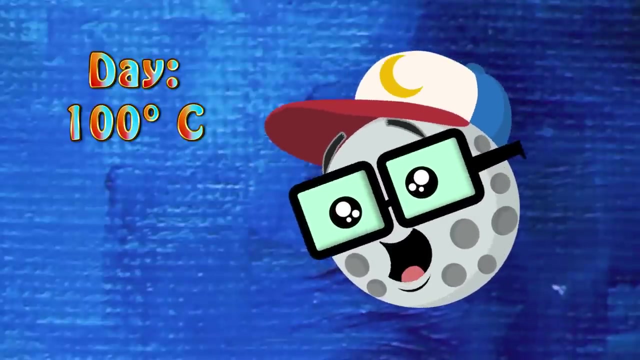 What NASA? That's the US space program. You better ask NASA for a rocket ship too. Oh right, And I'll learn to fly it. Oh yeah, Sure, you can come visit, But I must warn you, I do get very hot during the day and very cold at night, Much hotter and colder than on Earth. 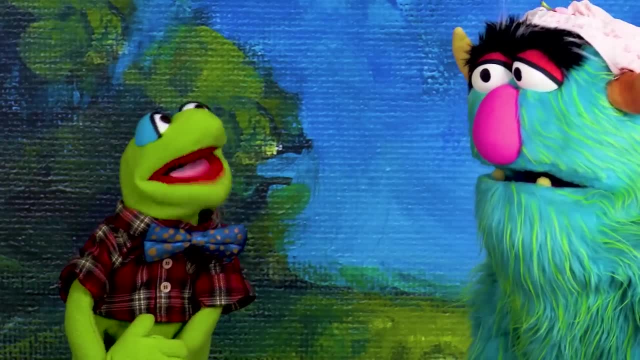 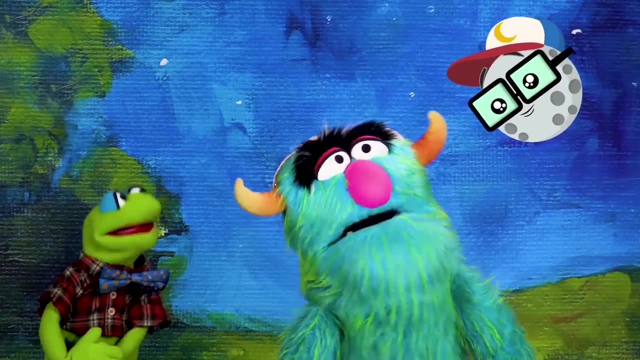 Ah darn. Yeah, you see, I only like nice weather, Plus uh, I don't know anybody that works at NASA. Well, you can always see me out at night. That's right, I'm bored. I'm going to see what's in my refrigerator.